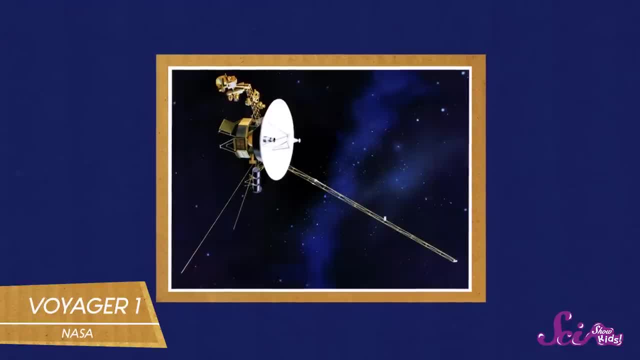 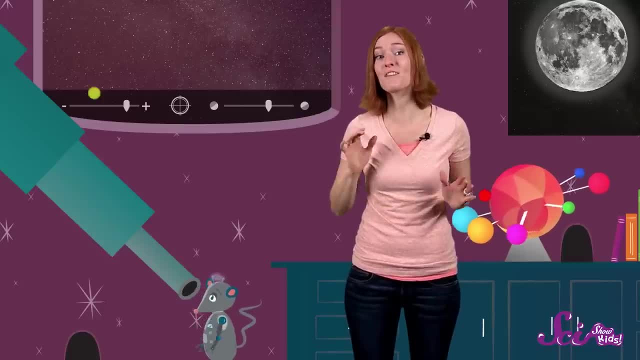 called Voyager 1.. It's a probe about the size of a small car but doesn't have any people in it. It has flown from Earth through the solar system, taking pictures of lots of the planets as it went, and it took over 35 years to reach the edge. It's so big. 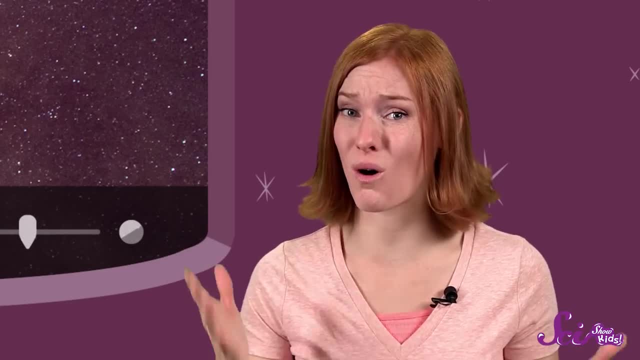 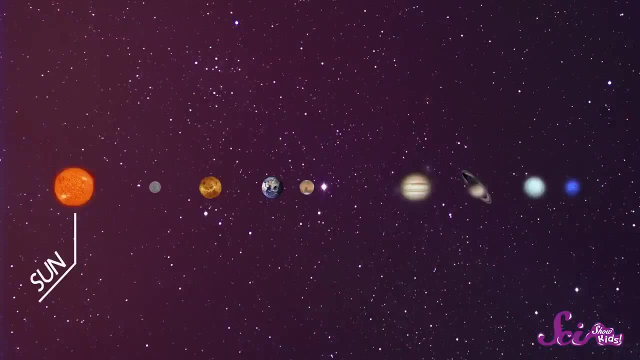 that today we're just going to cover half of it. And keep in mind it took Voyager 1 all that time to fly from Earth, and Earth isn't even at the middle of our solar system. The Sun is. so let's start there, right at the 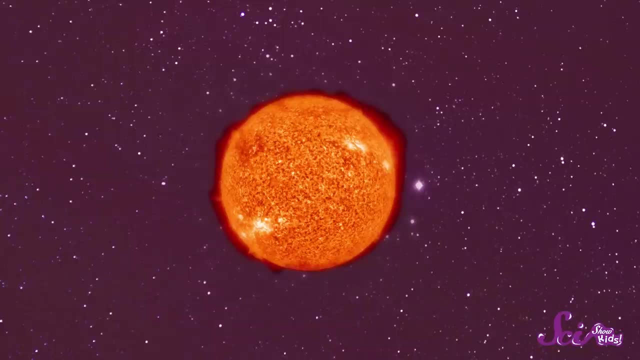 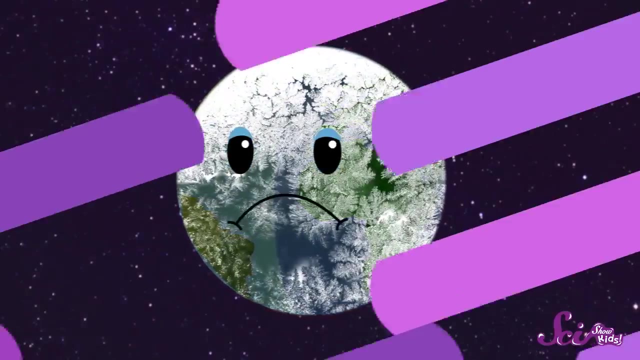 center of the action. The Sun is a star and like most stars, it's a huge ball of super hot gas that gives off light and heat. Without the Sun, Earth would be a dark, frozen world with no life. But Earth isn't the closest planet to the Sun. That would be Mercury. 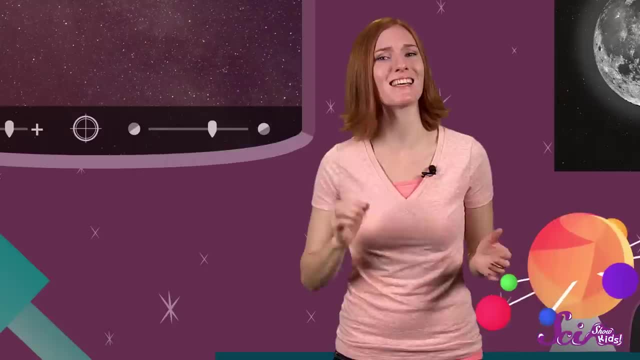 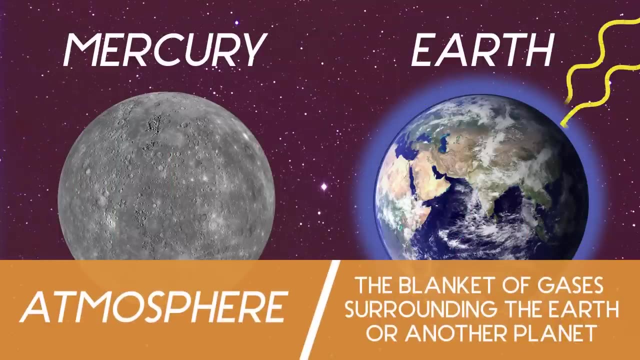 Not only is Mercury the closest planet to the Sun, it's also the smallest: It's less than half the size of the Earth. Mercury doesn't have a lot of gases around it like Earth does. Without these gases to hold in heat, Mercury has the biggest changes in temperature of any of the planets It can. 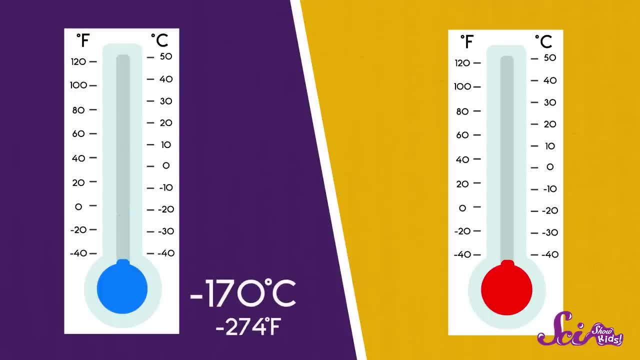 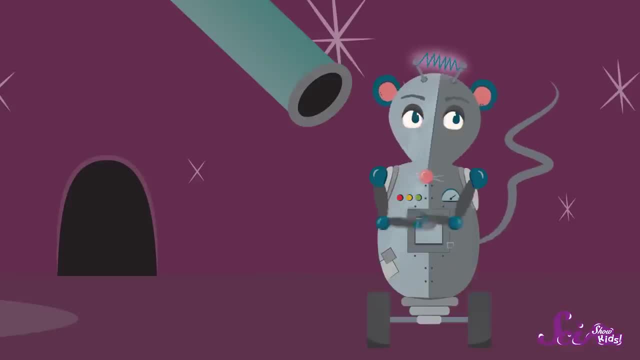 go from a super-chilly 170 degrees below zero at night to a very warm 425 degrees Celsius during the day. People couldn't survive on Mercury, and I don't think robotic rats could either. And things get even more extreme on Venus, the next closest planet to the Sun, Venus. 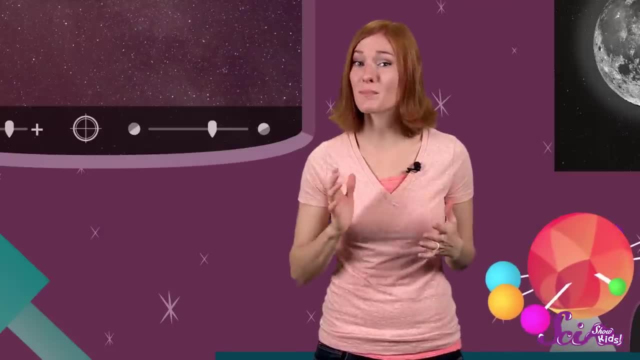 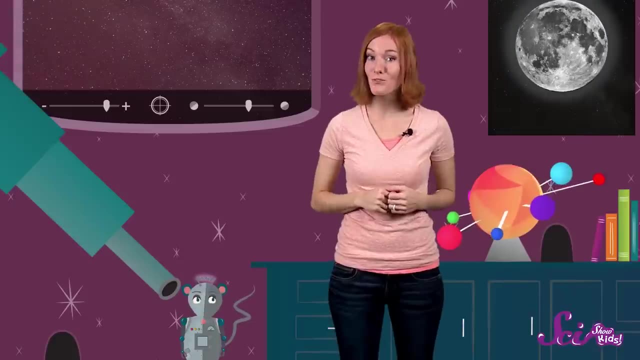 is the brightest planet in our solar system. If you know where to look, you can sometimes spot it from Earth Just after the Sun sets at night or just before when it rises in the morning. We've sent probes to Venus to take pictures too. They show us that the planet is rocky. 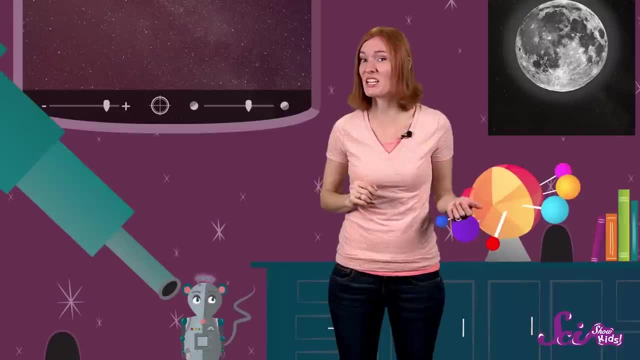 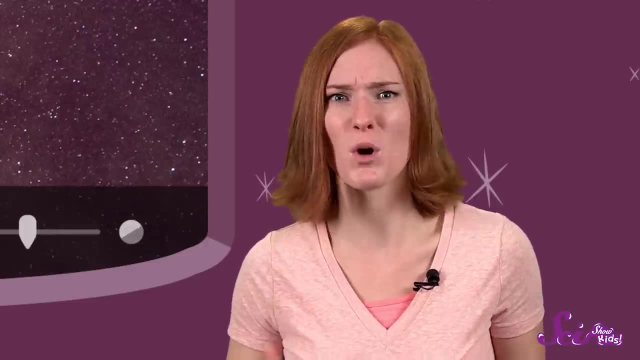 and covered with thick clouds, but doesn't have any life on it, because Venus is extremely hot. In fact, even though it's not the closest to the Sun, Venus is the hottest planet in our solar system, with temperatures reaching as high as 460 degrees Celsius. 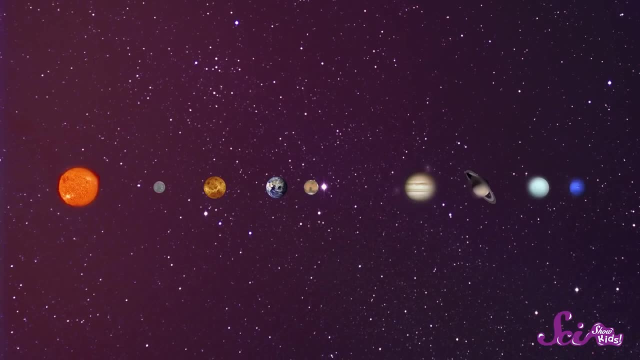 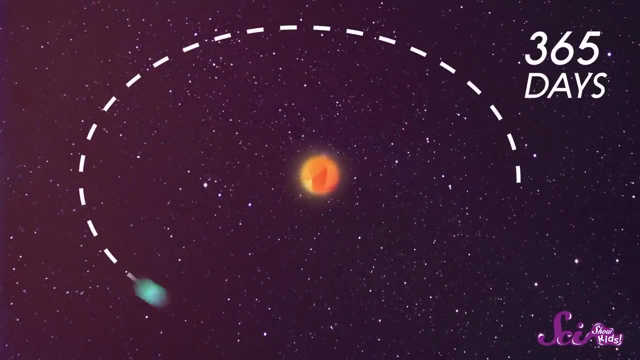 Whew, Let's cool off and head to the next planet. Hey, this place looks familiar. Welcome back to Earth. Earth is about 93 million miles away from Earth and it's the closest planet to the Sun. It's 93 million miles from the Sun and it takes 365 days our year for the Earth. 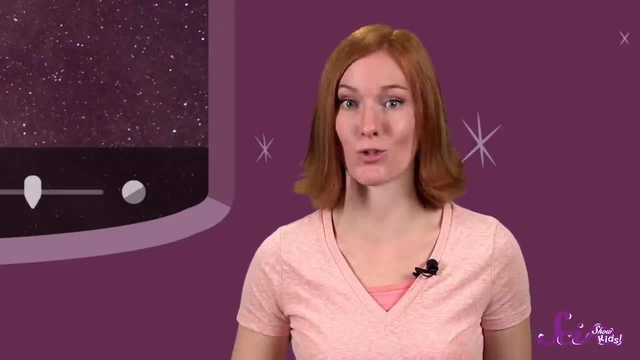 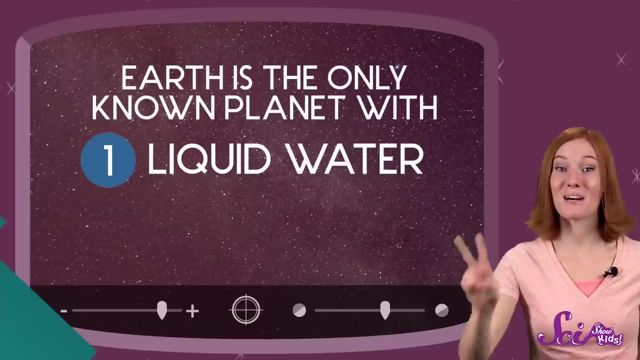 to orbit the Sun. And Earth is unlike any other planet in our solar system for at least two reasons: Number one, it's the only planet that we know for sure has liquid water on its surface, And number two, it's the only planet that we know has life on it, No other planets in.